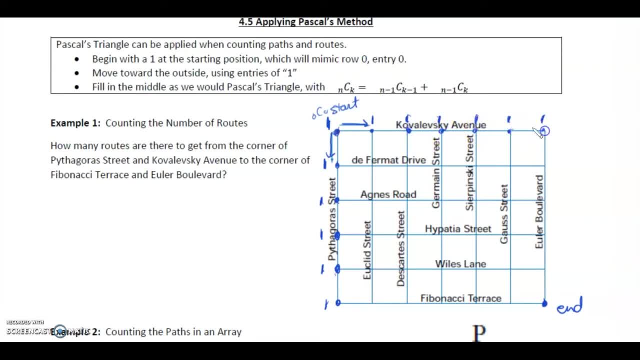 means these points. Okay, then what we're going to do is we're going to move toward, toward the middle, and we're going to be adding these outside numbers with our original equation there. So we learn this in 4.4 section, Okay, and we're going to fill up the middle and eventually get to the end. So apply to. 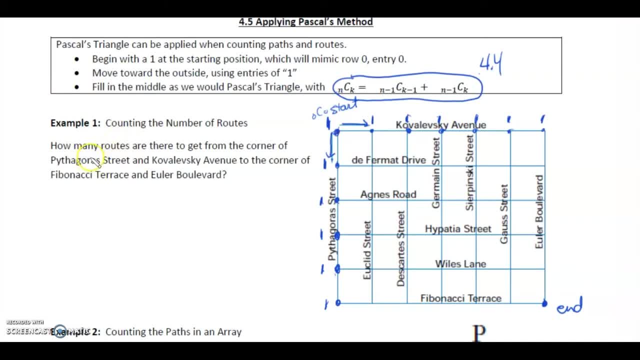 a question, example one, counting the number of nodes, and then we're going to add the numbers to be adding these in the middle Ready. So the first link in insert here is going to be a Tw ignorant group, And then we need the number of nodes to be in the first one. Okay, and that's the. 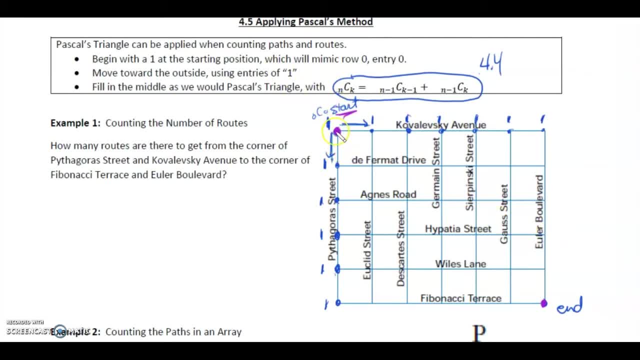 number one, non and then column, and it is down here. So it is . sw four. elite value s ▕ � s at i t s g s q p sets slopes states ?? Okay, so there's the problem here. We're going to say that this whole term is going to be 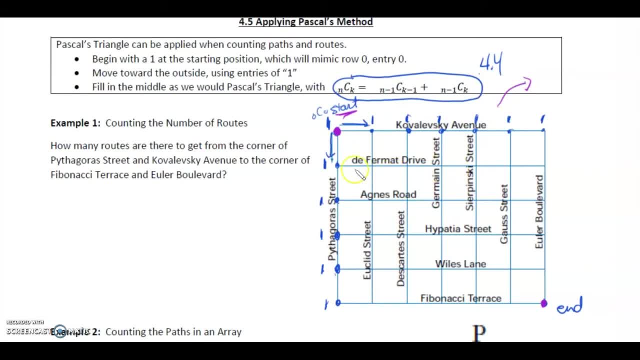 a number of "- North North ox, Redox, taper trabajo, North abilities like this way you'll be able to see the triangle, okay, and then get to this intersection. there are two routes and I'm going to give you an example: one route to the right one, and then down and 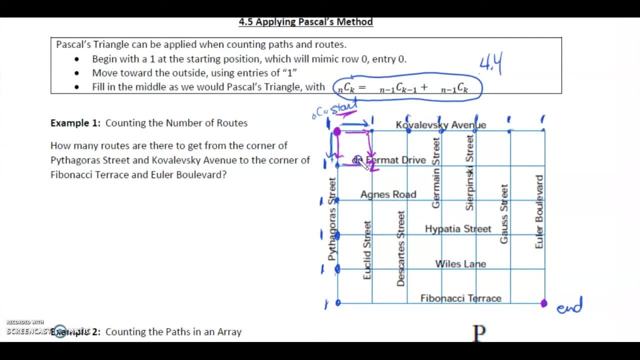 that's one route, and the other route is down and then to the right. so there are two different ways to get to furmat and euclid. okay, and then let's continue to go. so one plus two is three, and then two plus one is three. so I'm going to do one more explanation and then I'm going to say: 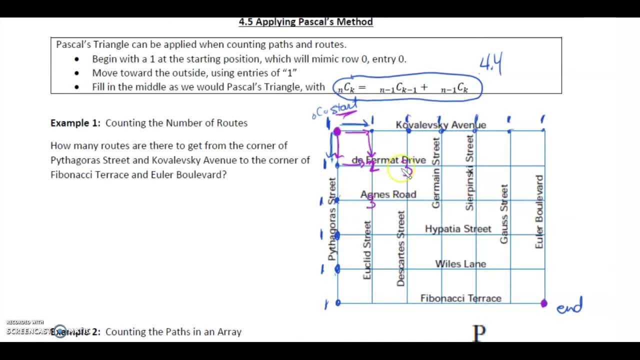 like we're going to assume that the the pattern continues. so for this street here. how can we? what are the three ways that we can get to here? well, we can go all the way over and then down. that's one way. We can zigzag, that's the second way. or we can go down and then all the way over. 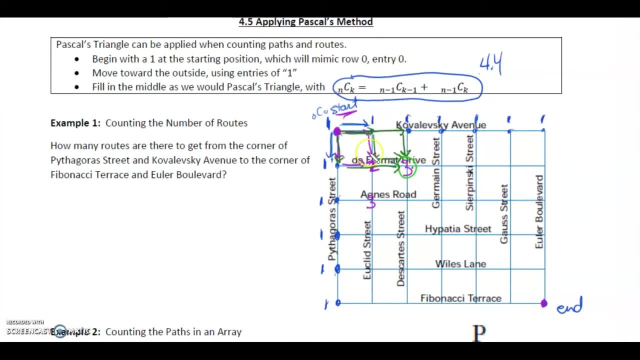 and that's the third way. Okay. so let's keep going: 1 plus 3 is 4, 3 plus 3 is 6, 3 plus 1 is 4.. Let's keep going: 1 plus 4 is 5, 4 plus 6 is 10, 6 plus 4 is 10, 4 plus 1 is 5.. Let's 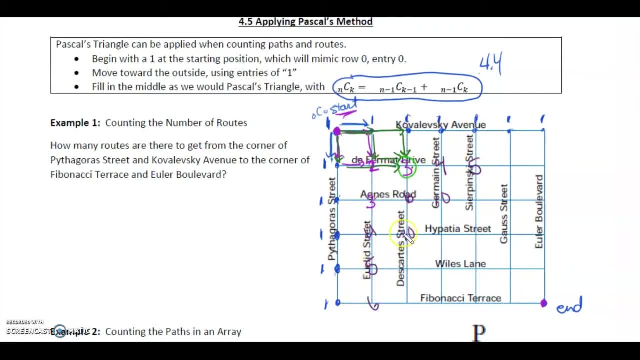 keep going. 1 plus 5 is 6,. 5 plus 10 is 15,. 10 plus 10 is 20,. 10 plus 5 is 15,. 5 plus 1 is 6.. Now I'm going to slow it down right now. So all of those were just from like. 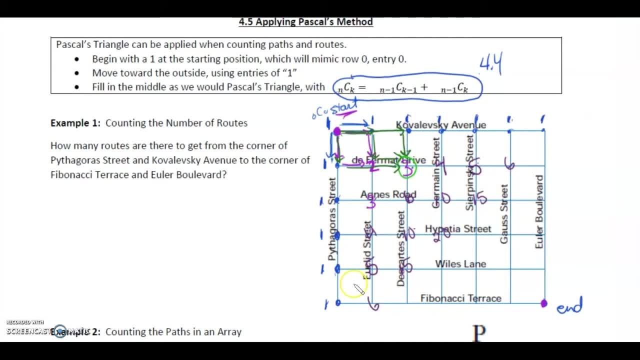 all of these numbers are from the original Pascal's triangle. Here's the difference. now We no longer have a root here, down to like a 1, so we're not adding this to it. So now it's almost like we're cutting off some of Pascal's triangle and just use 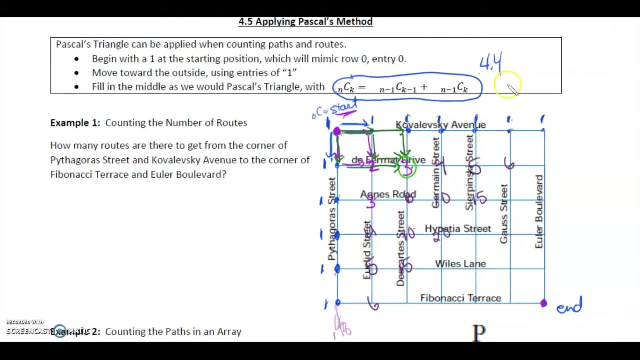 what you have here. So don't take shortcuts, don't use this, this formula every time, Like don't count how many rows to the right and down and then plug it in. It's not going to work like that. You have to go through the steps. So 6 plus 15, I get 21, and I'm doing. 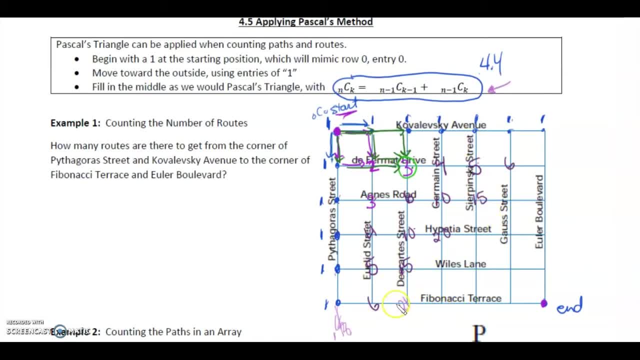 this with like a lighter color. I want to be able to see it. Okay, 15 plus 20, we get 35.. 20 plus 15, we get 35.. 15 plus 6, I get 21.. 6 plus 1, I get. 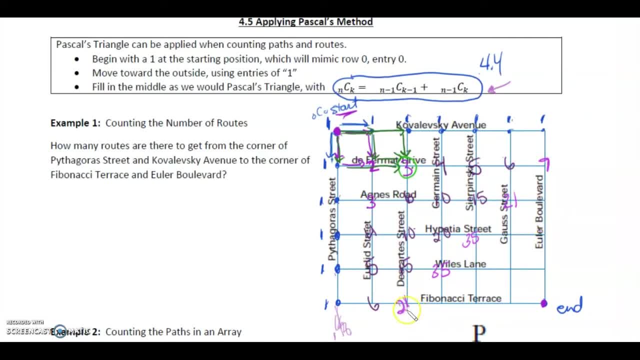 7. Okay, 21 and 35,, I get 56.. 35 and 35,, I get 70.. 35, 21,, I get 56.. And 21 and 7, I get 28.. Okay, 56 and 70,, I get 126.. 70 and 56,, again I get 126. And then 56 and 28,, I get 84.. So 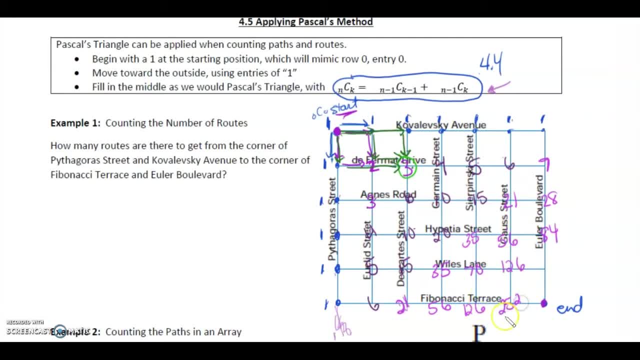 126, and 126 is 252.. And then 126 and 84, I get 210.. So finally I get 400,, oops, 462.. So there are 462 roots to get from. let's just call it start to end, Right, It could be A to B, start to end. Start to end. 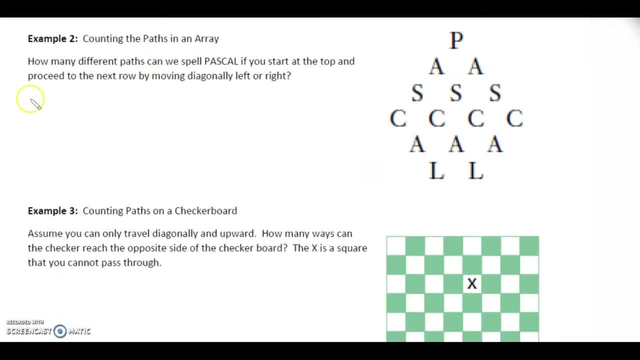 Example two, counting the paths in an array. So how many different paths can we spell, Pascal, if you start at the top and proceed to the next row by moving diagonally left or right? So all this means is that, like we're going to start with P, So there's one. 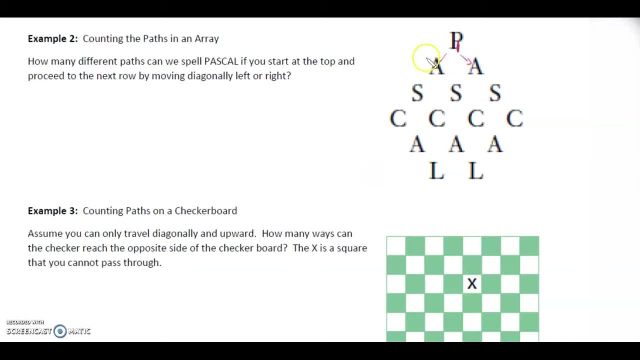 way to write P, and then we branch out, And there's one way to write PA, and there's one way to write PA. Now we branch out And I'm going to put ones down the sides. okay, At this point I'm going to go one plus. 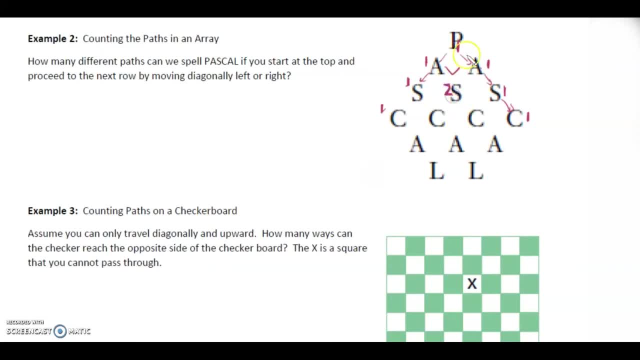 one gives me two, So we can either go PAS this way or PAS this way, And then one plus two is going to equal three. So again: PASC, PASC or PASC. Okay, So there's three different routes to get to this C value, And there's three different. 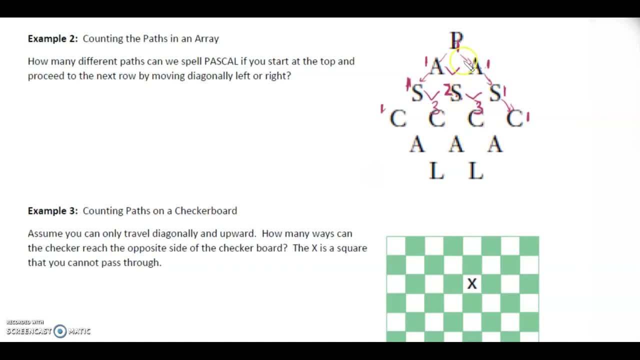 routes to get to this C value. And now, this is when the Pascal's triangle changes. Okay, Because we no longer have the triangle going out all the way, we have a tapering back in, So these are going to be different numbers. 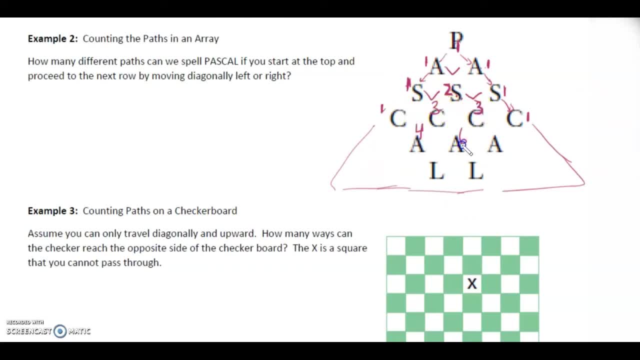 So one plus three is four, Three plus three is six, Three plus one is four, And then four plus six is ten. Six plus four is ten. Now, if we don't taper back off to like one like one letter here, let's call it like letter. 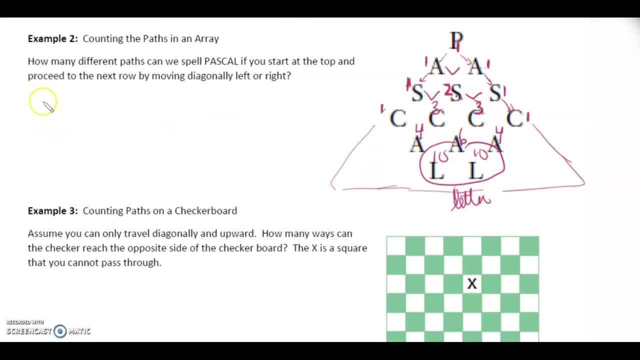 okay. What we have to do at the end is add these. So ten plus ten is twenty. So therefore there are twenty routes or twenty paths in this spelling of Pascal. All right, Example three: Counting paths on a checkerboard. 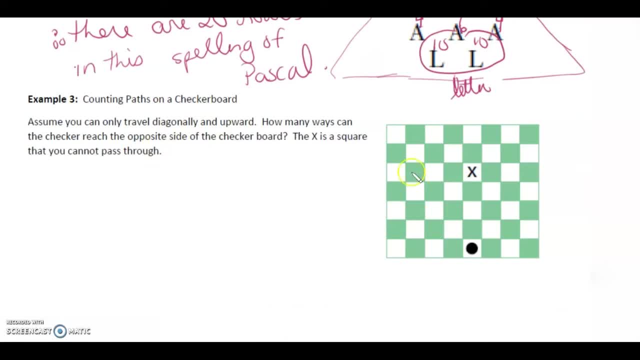 So assume that you can travel diagonally and upward. Okay, How many ways can the checker? so this is the checker with the circle. okay, Reach the opposite side of the checkerboard And then just note: the X is a square that you cannot pass through. 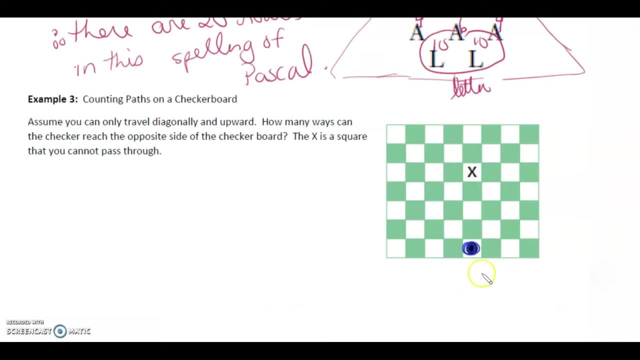 So we're used to flowing down, like from top to bottom, So now we're going to flow the other way. We're going to flow from the bottom to the top, So from here we would go diagonally, So there's one path to get here. 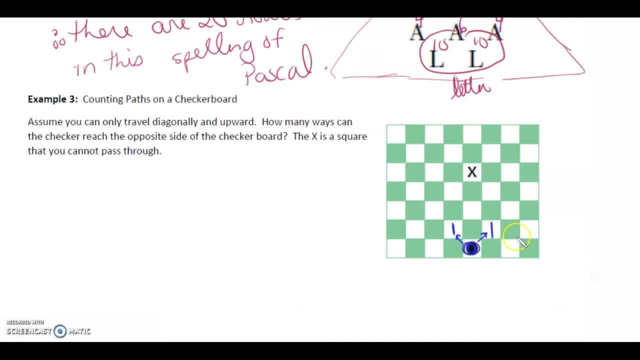 And one path to get here. Please note: we can never reach this square or this one or this one, because we're going diagonally upward, So diagonally left or right. Okay, let's go again. Okay. Example three: 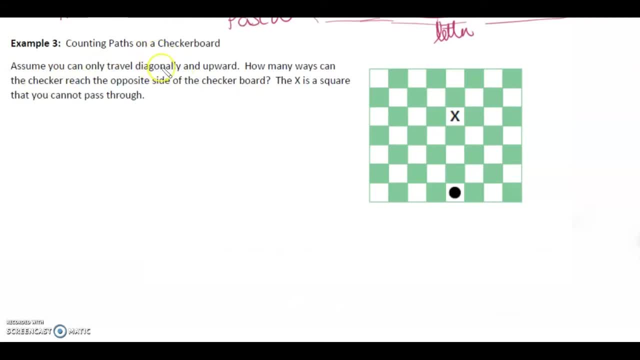 Counting paths on a checkerboard. So assume that you can only travel diagonally and upward. How many ways can the checker? so this is the checkerboard. Okay, So we're going to go to the checker here- Reach the opposite side of the checkerboard. 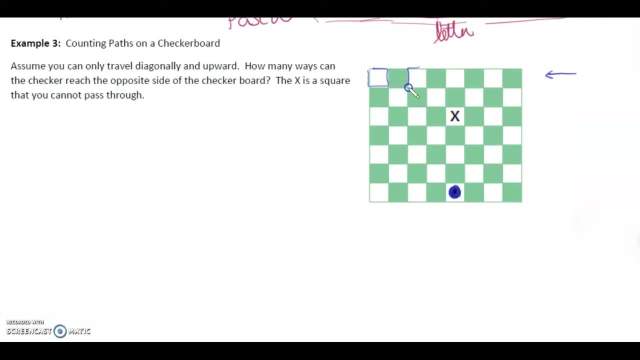 So any of these white squares here? okay, The X is a square that you cannot pass through. So that is the extension onto this question. okay, So for the checker piece, we want to move up the board. okay, So we've done all questions that we've moved down. 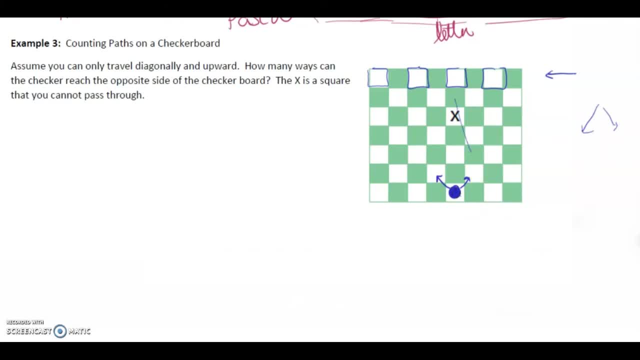 Try again. We've moved up the triangle, So now we're going to go backwards. We're going to go up the triangle, So not backwards, Upside down. Okay, So this checker can get here one way. This checker can get here one way. 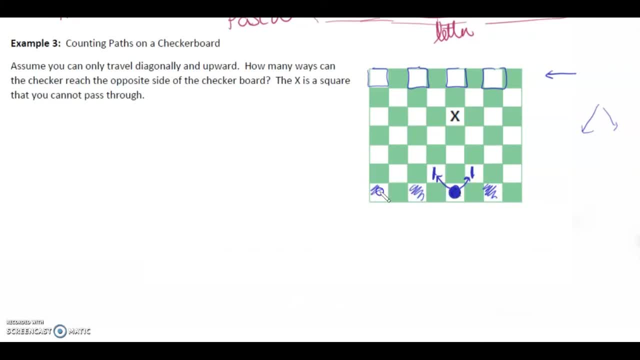 And we're never actually going to move backwards, So we're never going to be able to reach these squares. Now, the checker can move this way, one way and to this square, one way And again. Okay, So we're never, ever going to be able to go backwards. 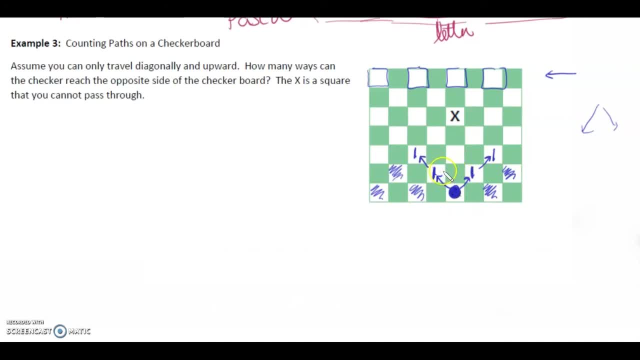 So we're never going to hit these squares. Now the checker: if we do, one plus one equals two. there are two ways that the checker can get to this square: One way, two way. okay, So let's keep going. The checker can get to this square one way. 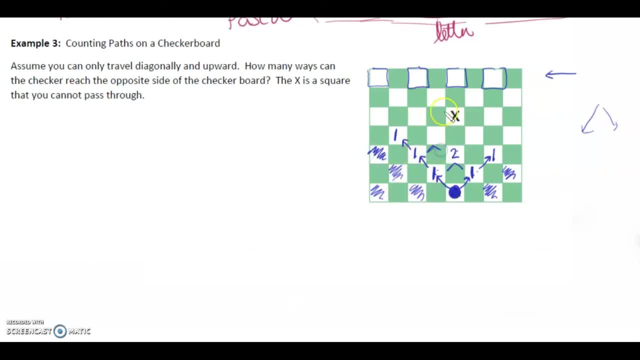 It'll never get to that square, Okay, And one plus two is three. Two plus one is three, And we just branch off one way to here. Okay, The checker can get to this square one way, This square four ways: One plus three. 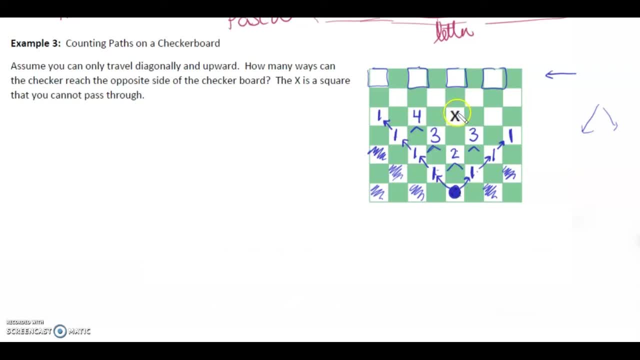 Now we cannot go through this. this X, So this is basically a zero. We can get to this X square Zero number of ways, So we'll just leave that there. It's not six. We can't land here, Okay. 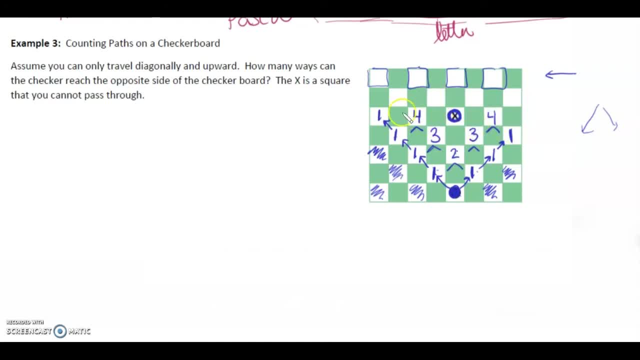 And then we have three plus one, which is four. Okay, We can get to this square. One plus four is five, Four plus zero is four, Four plus zero is four, And then this just branches to the right, Just like how we would do the ones all the way down, since this square only has the number. 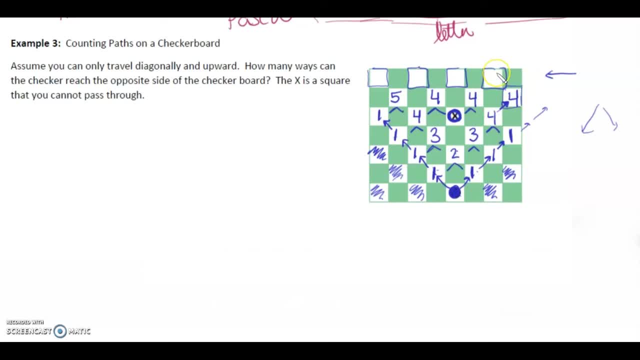 four like funneling into it, we would put a four. Okay, So this square only has the five funneling into it, So we go five. five plus four is nine. Four plus four is eight. Four plus four is eight.